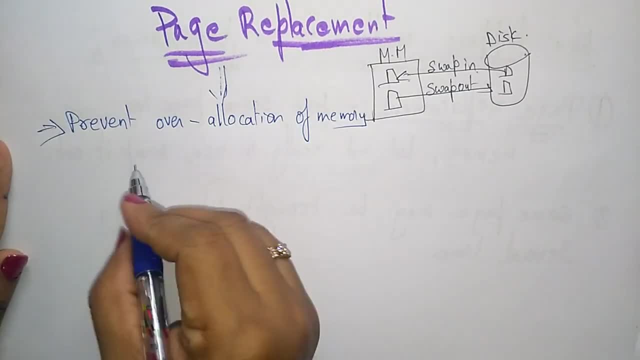 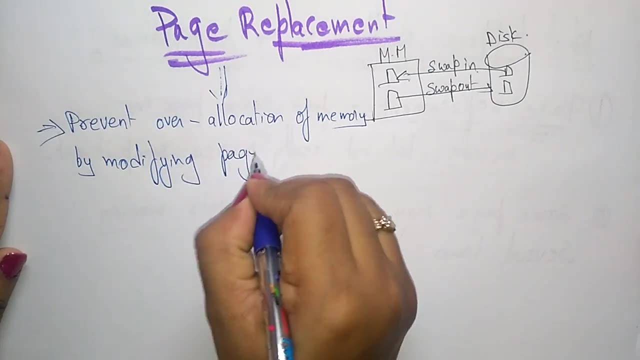 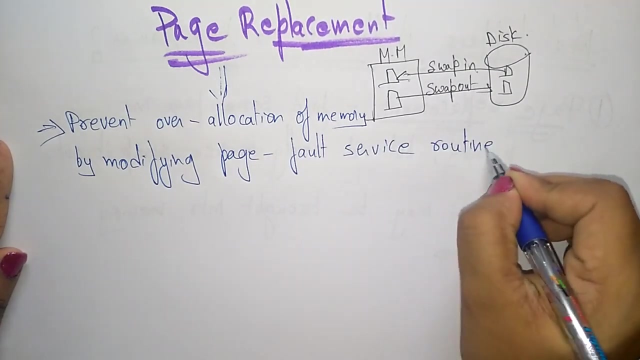 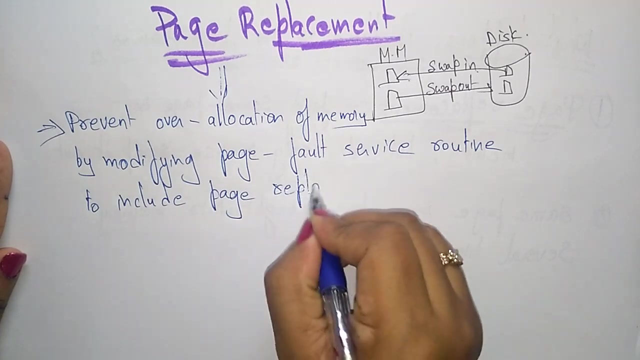 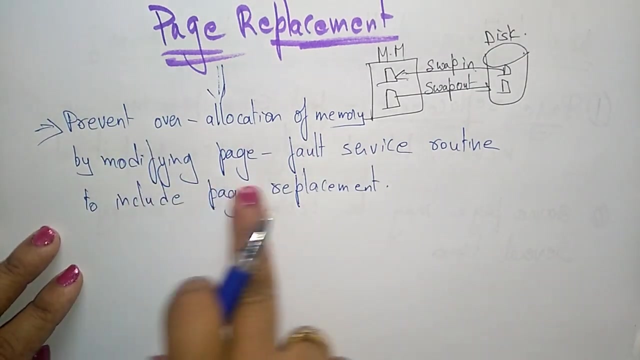 So to prevent the over allocation of memory by modifying modifying page fault service, page fault service routine to include page replacement. So for that reason we are using this page replacement to prevent the over allocation of memory by modifying the page fault service routines. 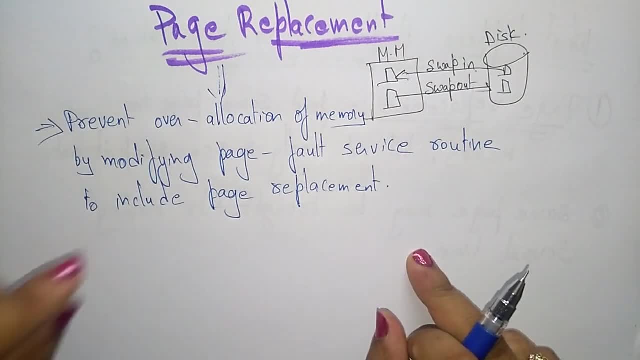 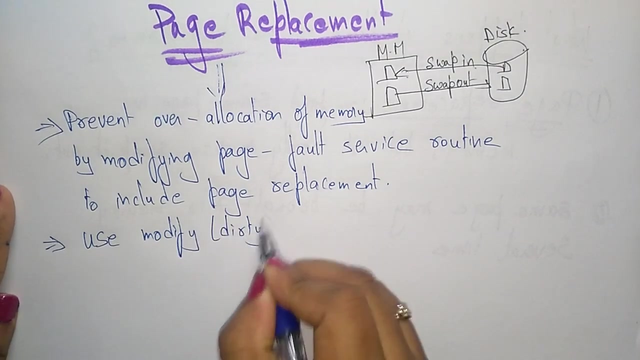 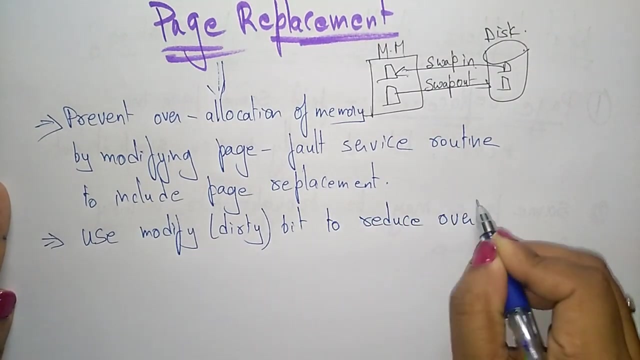 We have to include the page replacement. So in this page replacement we are just using the modified bit or a dirty bit to reduce the overhead of page transfers. Use modify bit, or you can call it as a dirty bit, So to reduce overheads of page transfers. 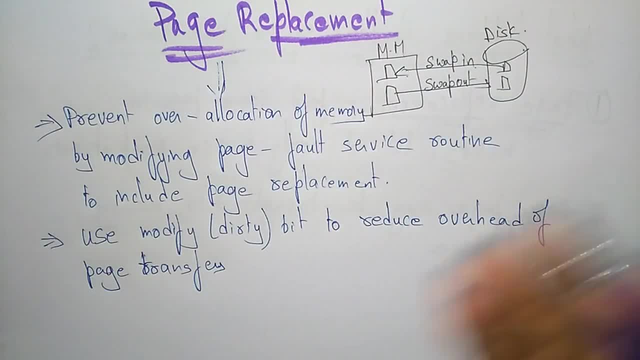 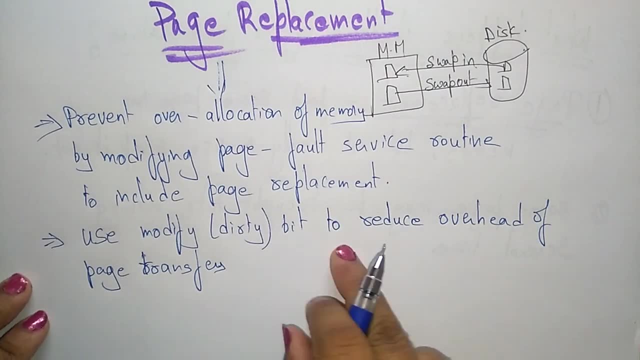 So every time swap in, swap out, swap in, swap out, it takes the overhead of the main memory. So to reduce that overheads of page transfers we use this modify bit or dirty bit in the page replacement So only modified pages are written into. 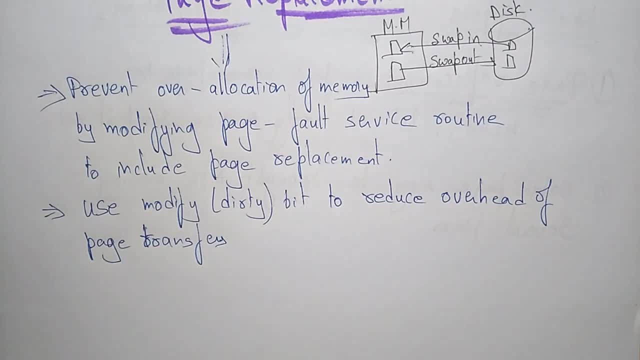 So this modified bit will, the dirty bit will be used. It indicates that only these pages are written to disk. So the page replacement completes separation between logical memory and the physical memory. So because the large virtual memory can be provided on a smaller primary memory. 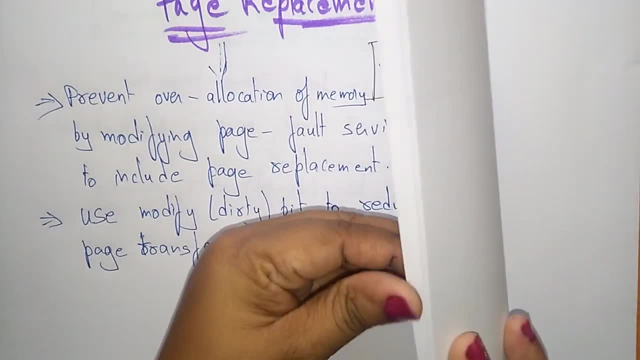 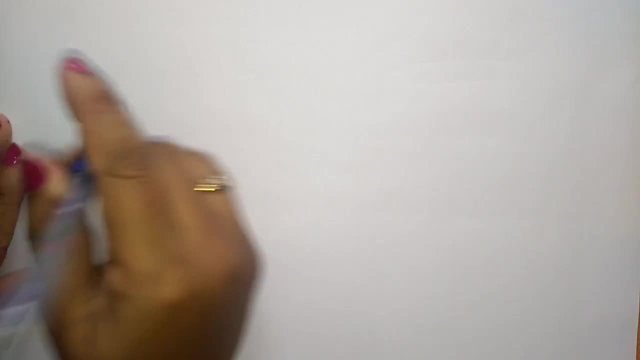 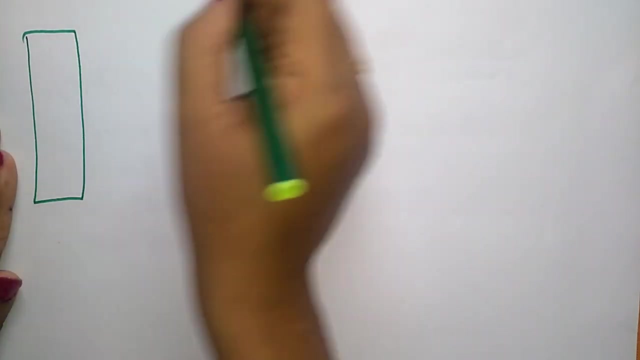 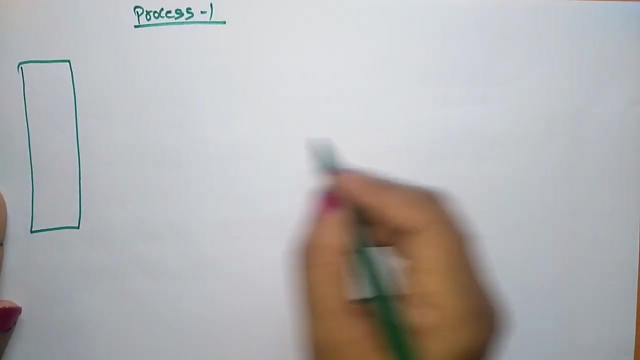 So let me explain the page replacement technique with a simple example, So how the page replacement will be handled. So let us take: so this is a page table. So here I am explaining the process one. So this is a page table. 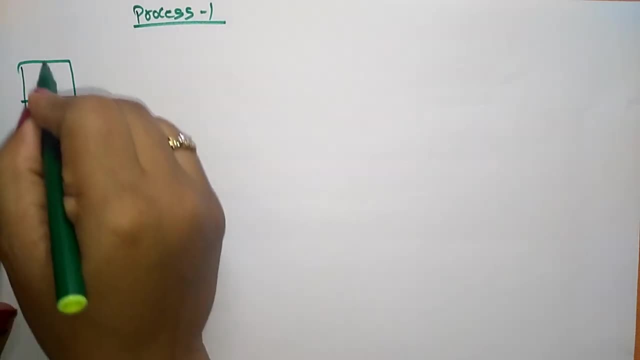 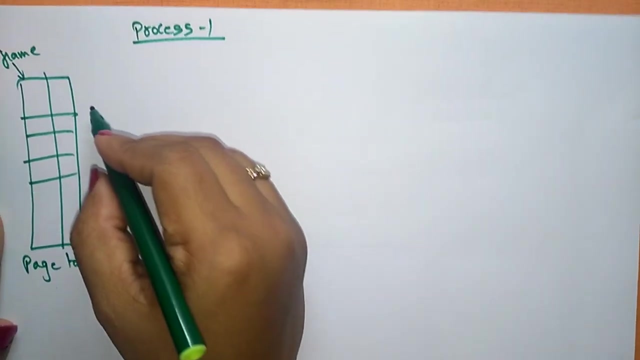 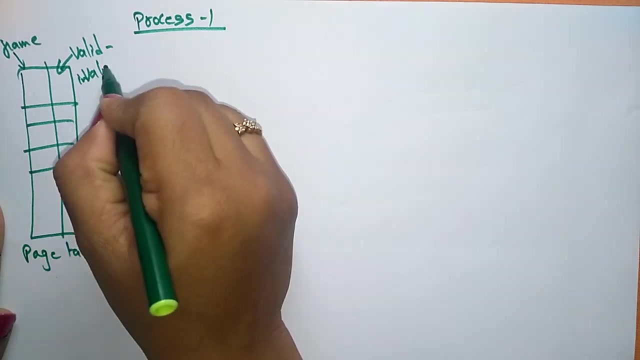 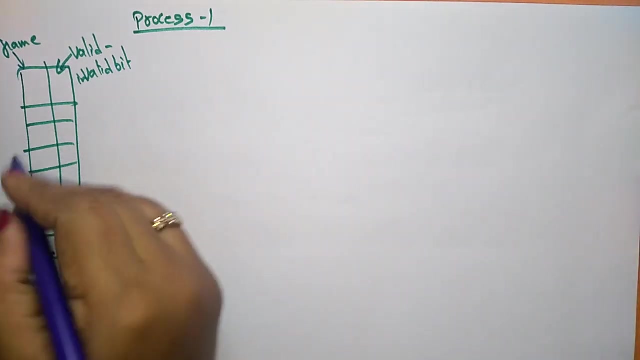 This page table consisting of frames. This is a frame, This first box is a frame And the second box indicates the valid or invalid bit. Valid or invalid bit. Okay, So here we are taking, suppose this is a 5.. 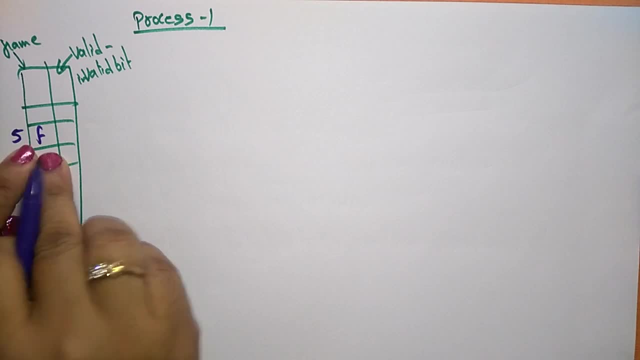 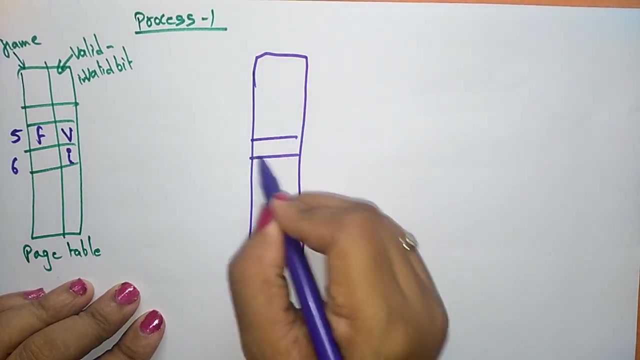 The 5,. okay, the 5 frame is a valid And the 6 is Invalid. So the 5 is present in the main memory and the 6 is an invalid, And here we are taking main memory. So main memory holds the victim. 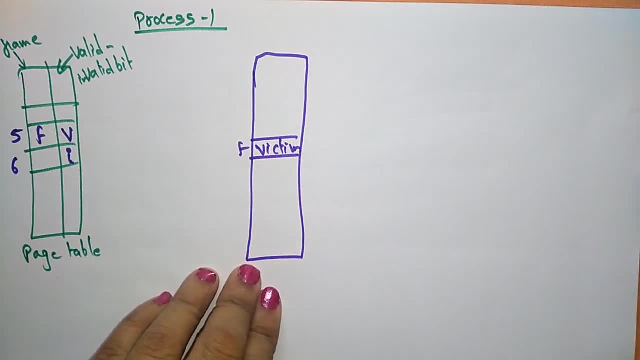 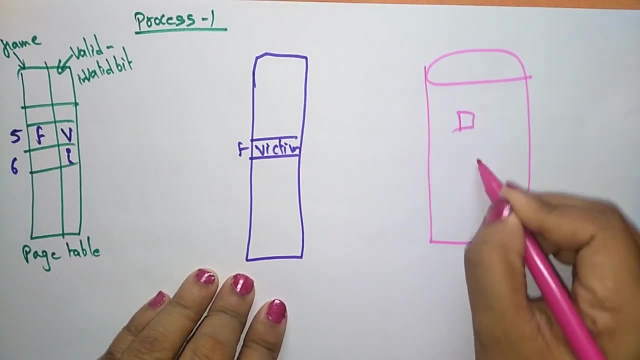 So that is a frame it is holding, And here we are having the secondary storage, That is the disk. The main memory is detail disk. Okay, So first the victim, the main memory. swap out the page. So now I am going to look at this. 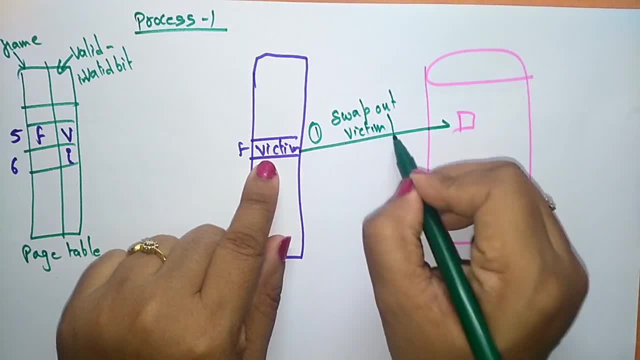 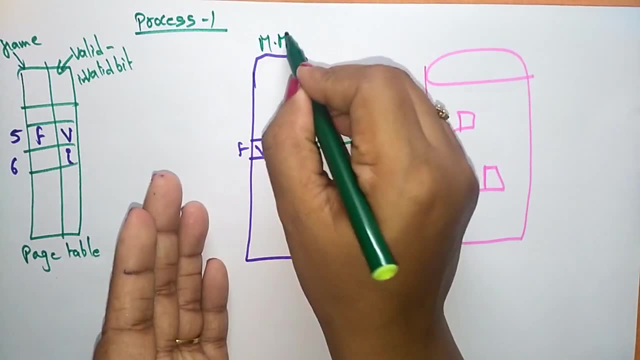 And here look at my detail data. so I am going to check the status of this page. So the main memory thought this page we are not using frequently, so we just swap the page. So the main memory is just swapping the page. This is the disk. 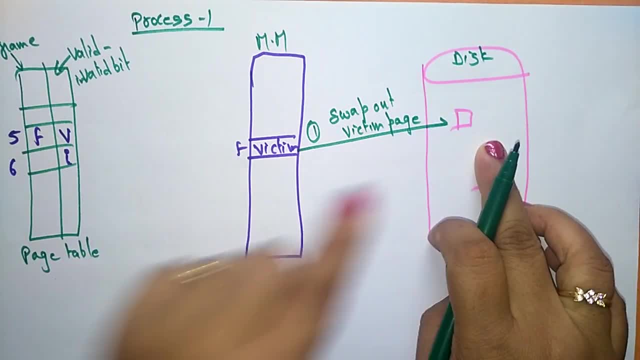 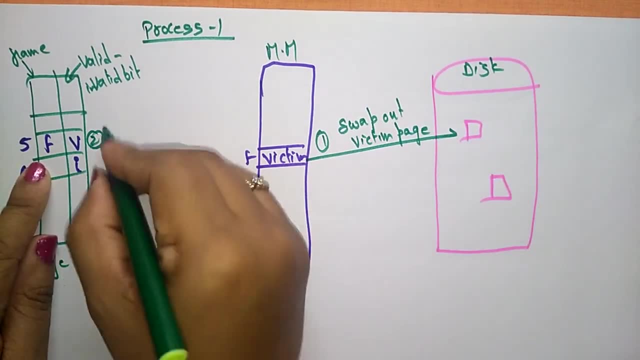 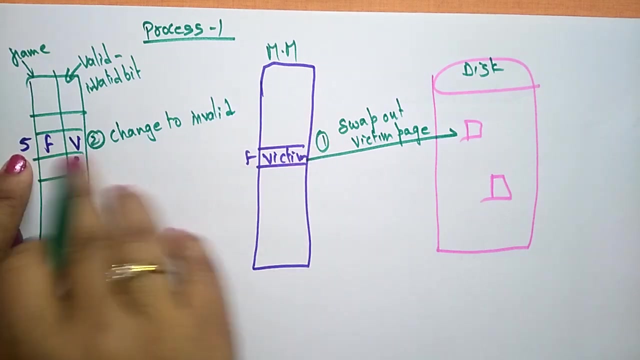 The main memory, swapping the page to the disk. So whenever I sub- Daddy to describe a table. so when will you do at first step the disk. now the CPU is demanding for the page. the second, it's changed to invalid. so because I'm just swapped the page to the disk, so whenever I swap the page to the disk, 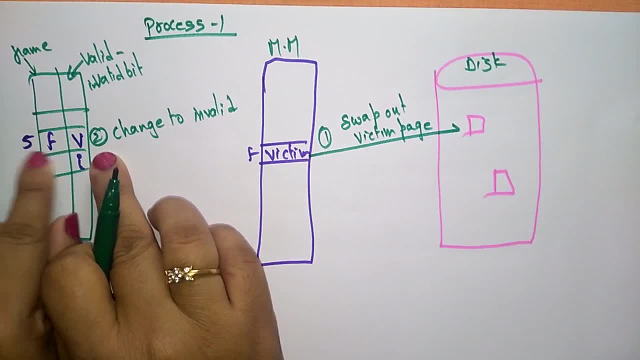 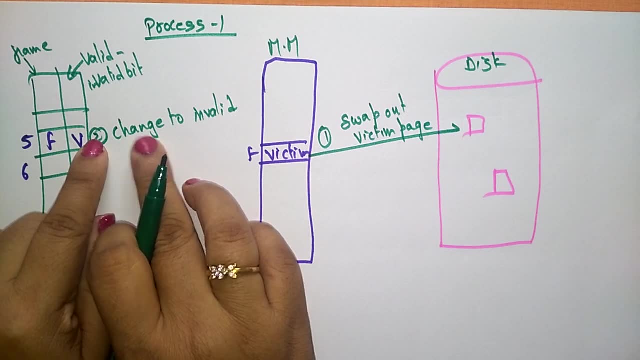 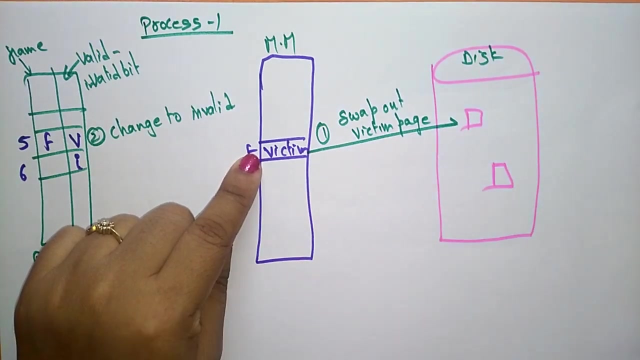 the CPU is asking for fifth page, fifth frame, so, but this is becomes invalid. so change this to invalid. so whenever it is changed to this invalid, the controller transfers. means because the pros, the CPU, identify the page fault. so whenever the CPU identify the page fault, the controller 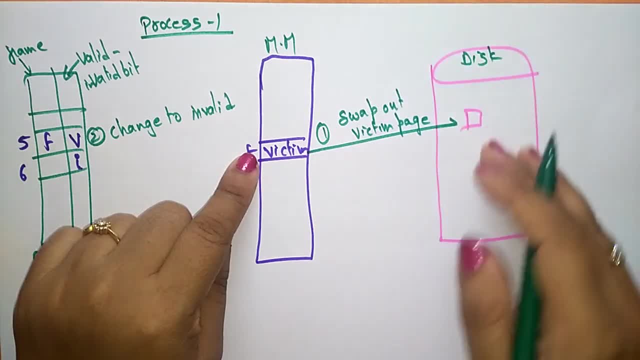 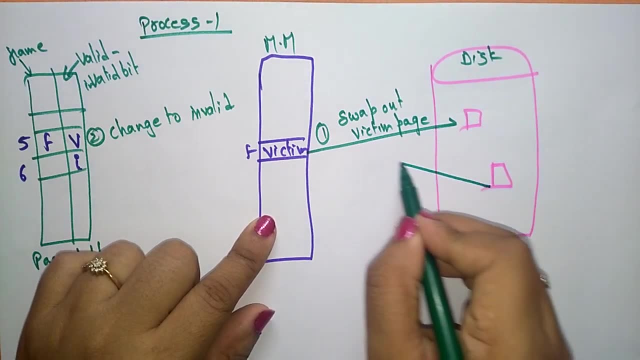 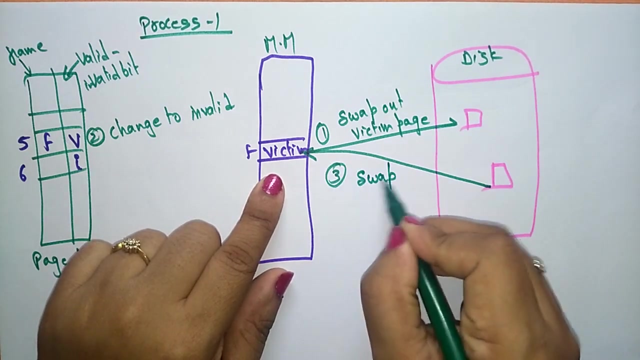 transfers to the operating system. now the operating system is send the request to the disk and take the page that is already swapped out to the disk and came back and placed in the main memory. that is a swap div, the desired page. the desired page in the swapped desired page is placed here. ok, so 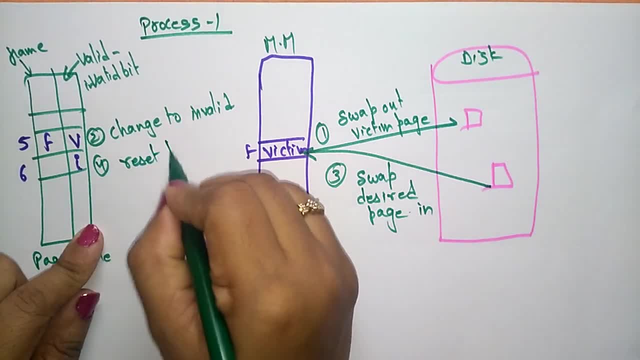 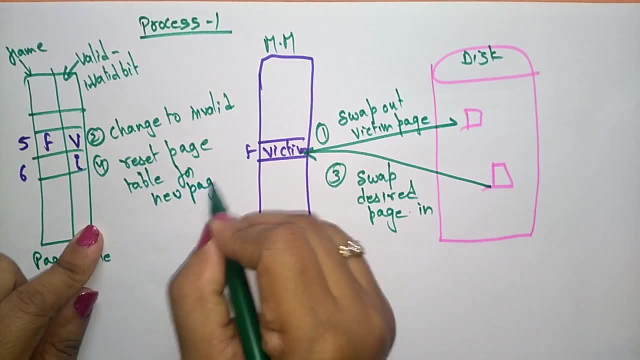 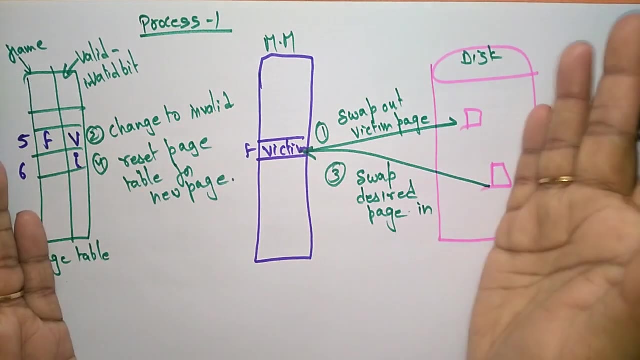 then fourth, reset page. reset page table for new page. ok, so here, up to here, we are just the CPU requested for page that is already swapped out and that page is placed in the the main memory. so whenever it is placed in the main memory it asking the page. 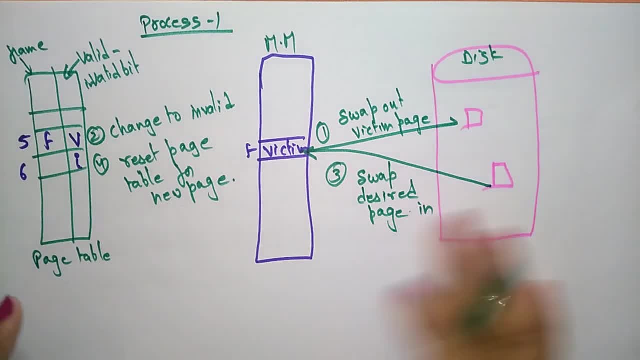 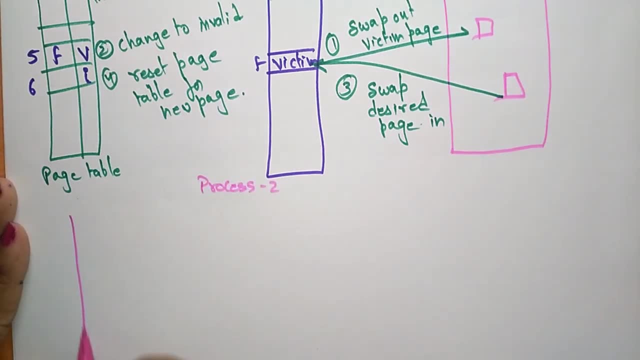 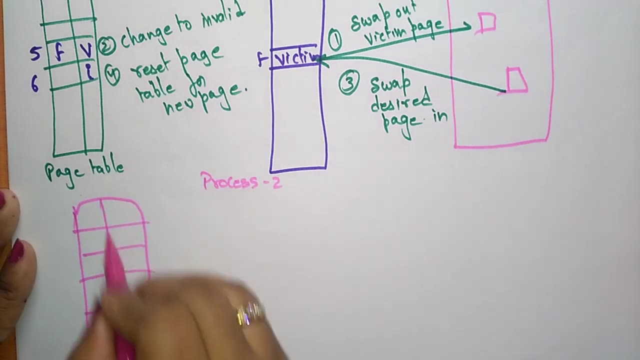 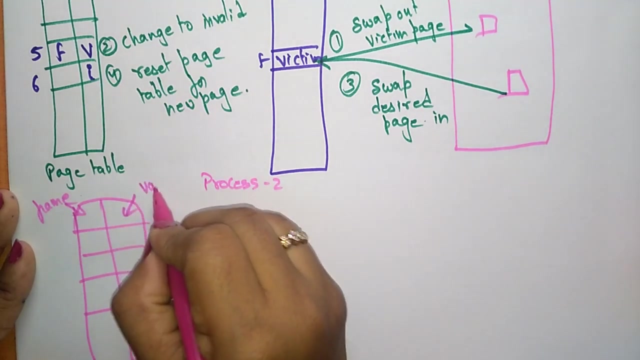 table to reset the page for new page. so now let's see the process to so, after resetting, how the page will be look like. now let us see. so this is a frame and this column indicates valid or invalid bit. okay, and this is a five. let's take. 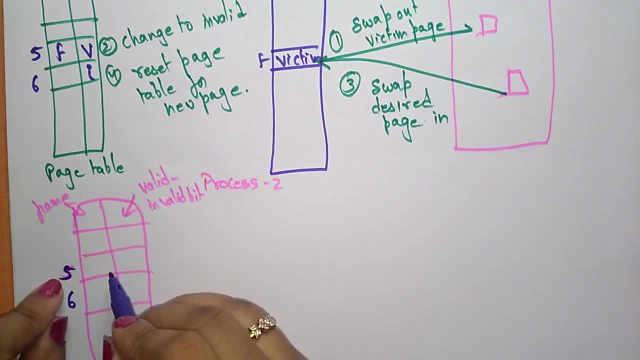 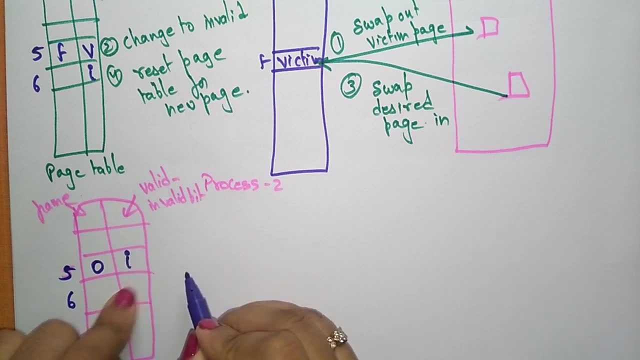 this is five and six, so the five is wrapped out, so zero, and it indicates invalid. okay, and this is a six. that indicates the frame. the new frame is added and this is valid because i reset the page table. so whenever i reset the page table it becomes like this: 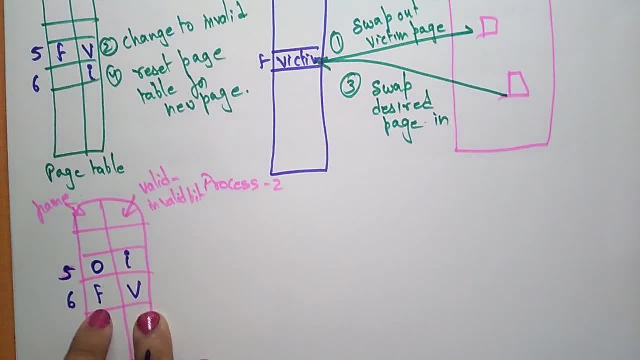 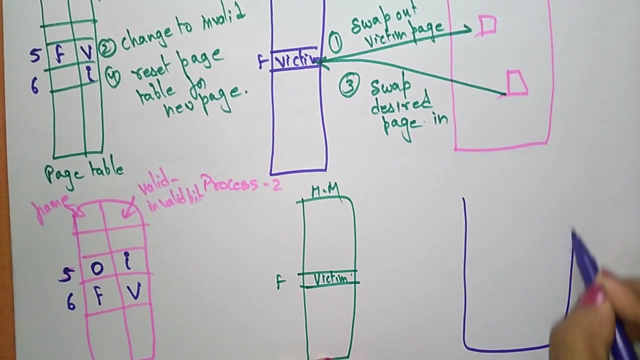 so the five indicates the zero and invalid and the new frame is added, the whatever the requested page f, v that is stored in the sixth frame and here this is the main memory victim and this is the disk. so, after resetting the table, so this disk holds the five and 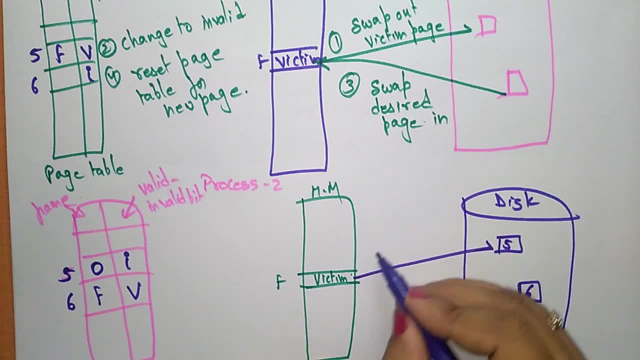 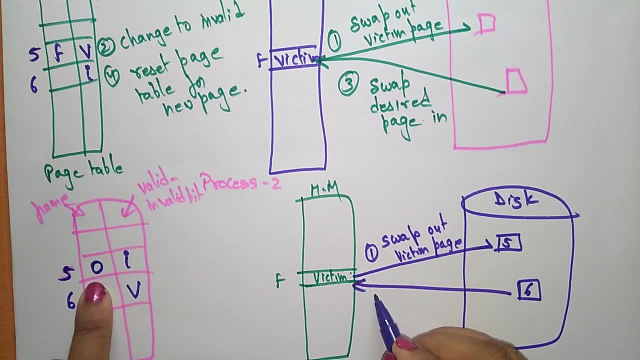 six, so the five is swapped out. so this is because this is invalid, zero indicating swap out, victim, victim. and this is the disk. so after resetting the table, so this disk holds the five and six, and requesting the new frame, that is a free frame, six, so this the two change to: 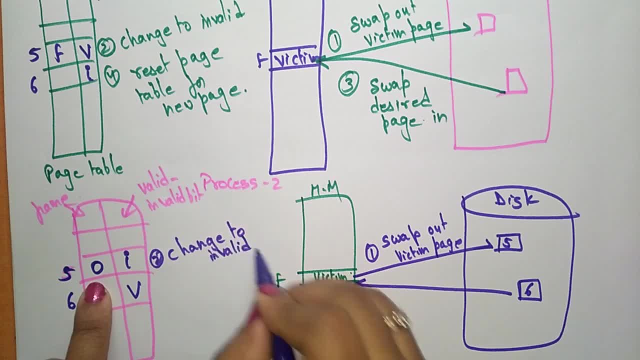 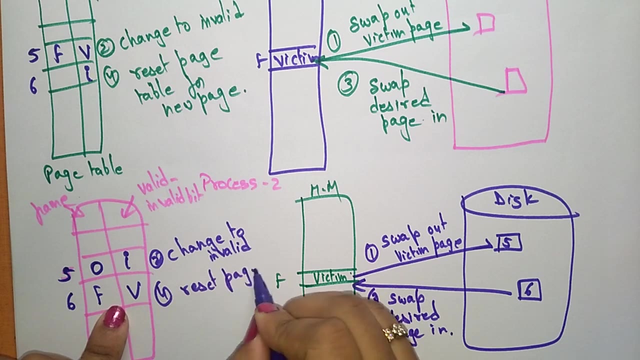 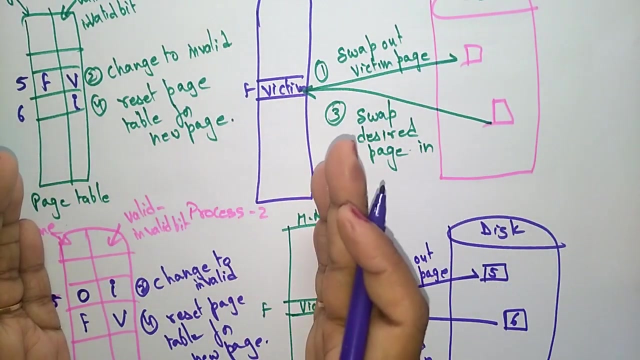 invalid. so the three swap desired page in and the fourth. so this is the new page. that is a reset page table for new page. so this is how this page replacement will be done. so whatever the page that we are swapped out, that page again will be placed in the main memory. so whenever it is placed, 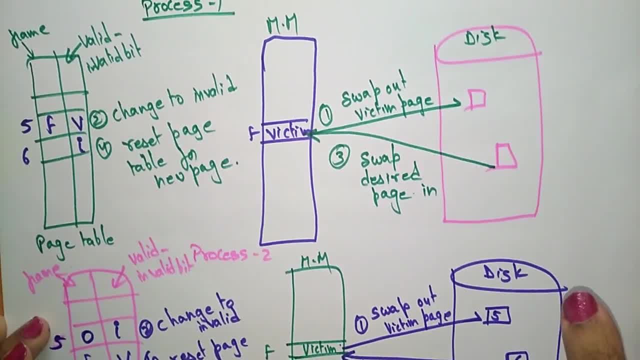 in the main memory. we have to reset the page table. so this is about the page replacements. so in the next videos i will discuss about the replacement algorithms. thank you,